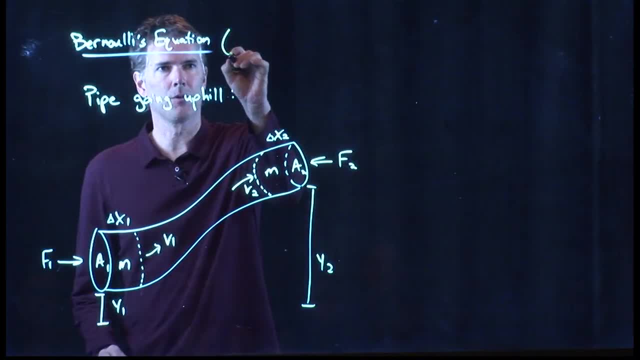 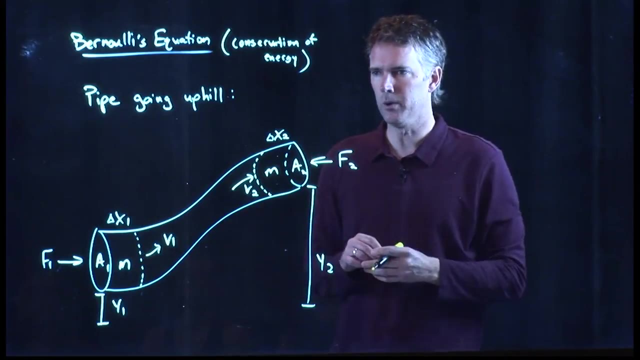 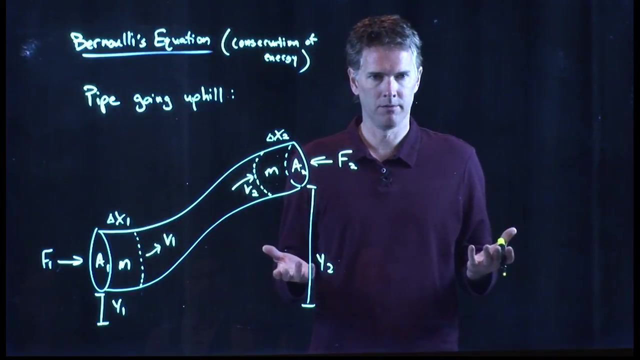 Bernoulli's equation is really Really not so complicated because it is completely analogous to conservation of energy. It's basically conservation of energy for fluids. So when you have fluids moving, you have kinetic energy. Anything moving has kinetic energy. When you have them going up a hill, you have gravitational. 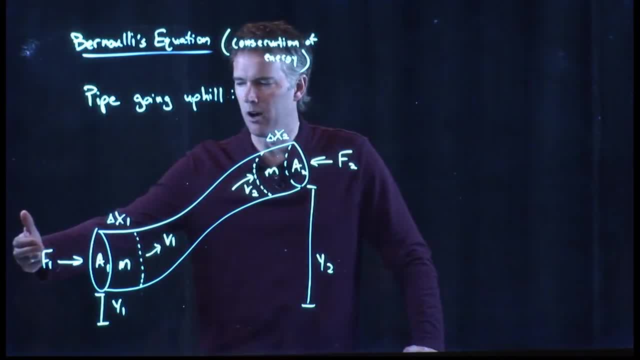 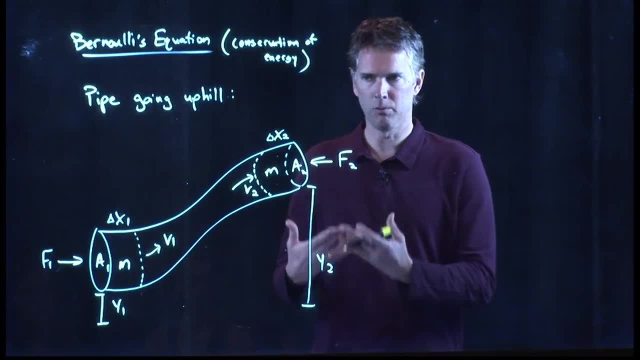 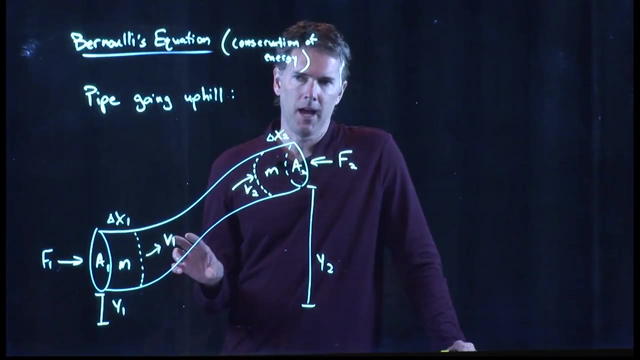 Potential energy. When you're applying a force, you're doing work. All of that stuff is energy, And so really, Bernoulli's equation is nothing more than conservation of energy. So let's set up the problem, And then we're going to skip a little bit of the math and we're going to jump to the solution. 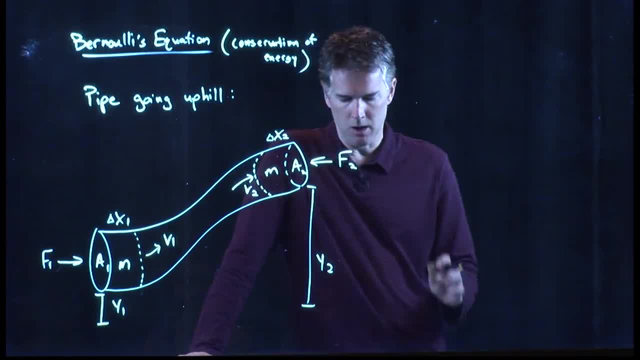 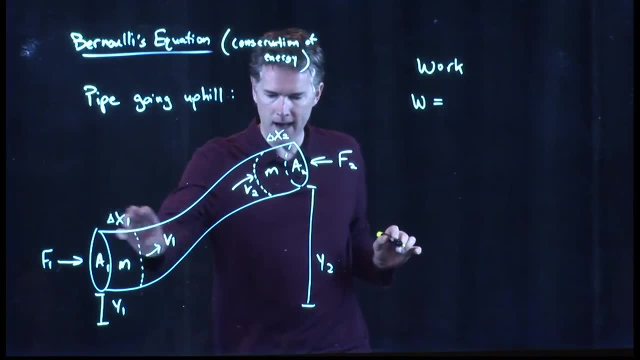 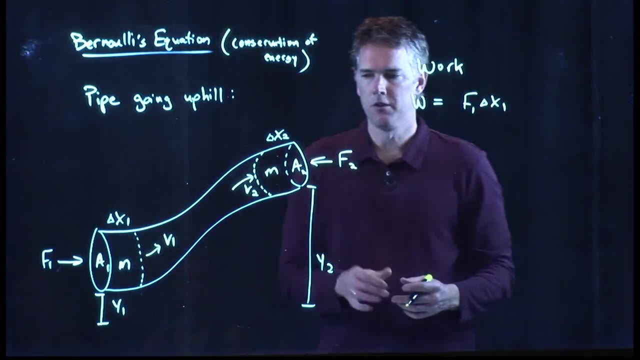 And then we'll see how we can apply that solution. Okay, the work involved in moving the fluid Is going to be what? Well, we have f1, delta x1. Pushing this fluid up. There's some work of this one trying to go the other way, but the fluid's still moving up. 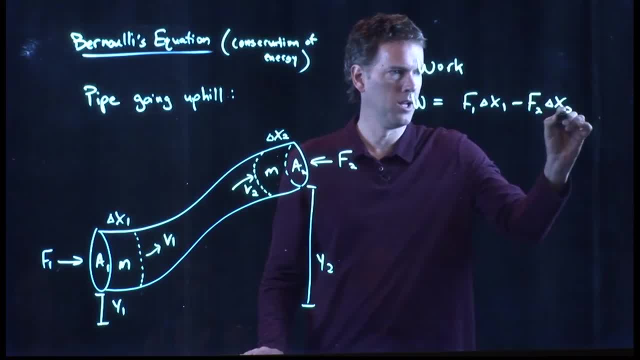 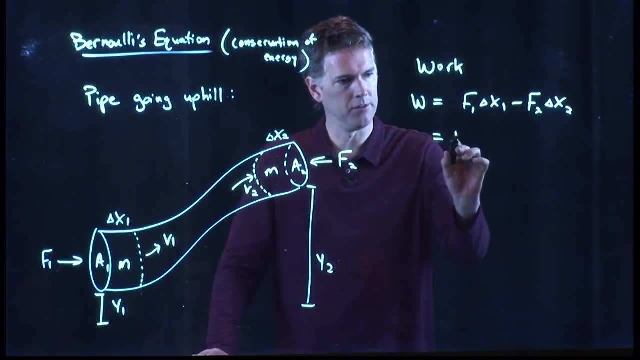 And so we have to make a minus sign: f2, delta x2.. All right, But we know that force relates to pressure. This is p1 times a1.. This is p2.. This is a1 times a2.. And a1 times delta x1. 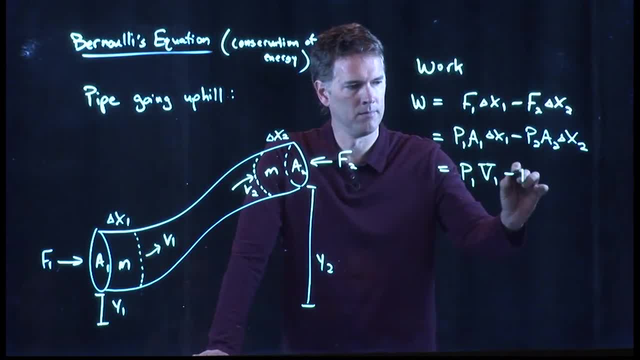 That is a volume: a2 times delta x2.. That is a volume. What's the volume of this fluid? What's the volume of this fluid Now, right off the bat. you should look at this and go wait a minute. 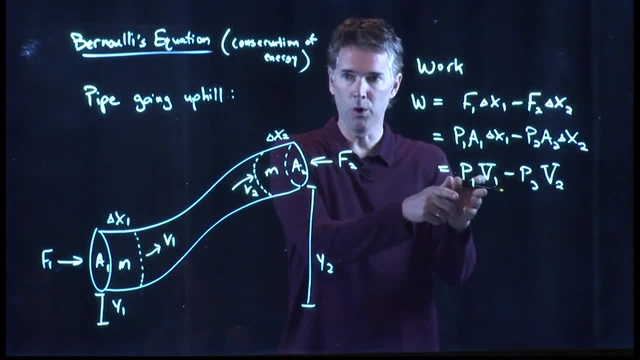 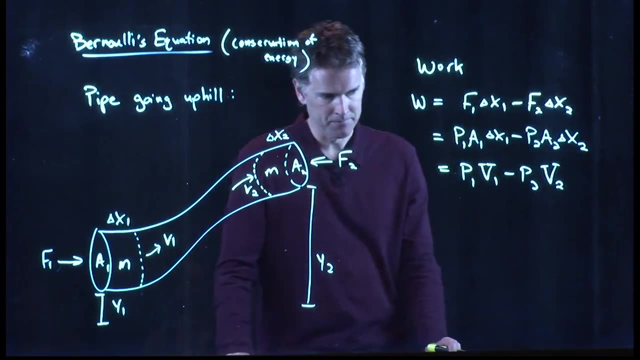 That sounds like something I learned about in chemistry. Chemistry Is this: f2 equals p, delta v, Right p times v. That is work, All right. So you might remember this from your chemistry classes, But the volume here is the same. 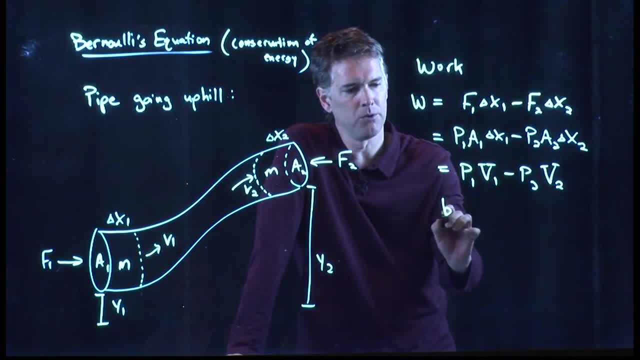 Right. The mass going in has to be equal to the mass going out. The density doesn't change, And so the volumes are in fact equal, And we will just define that as v And so work. And so the volume is equal to v. 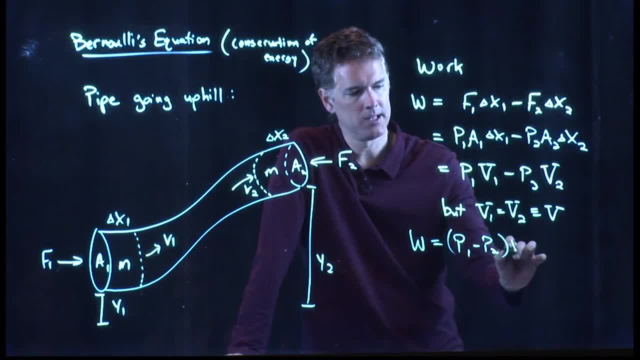 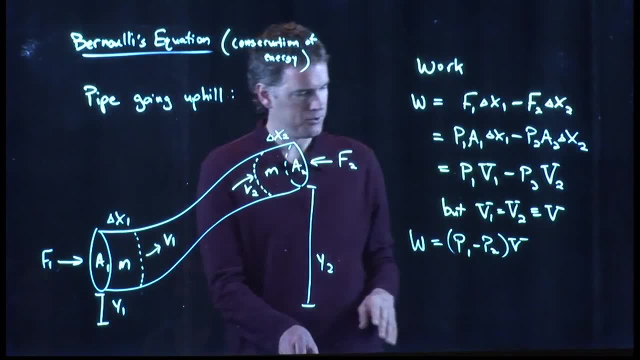 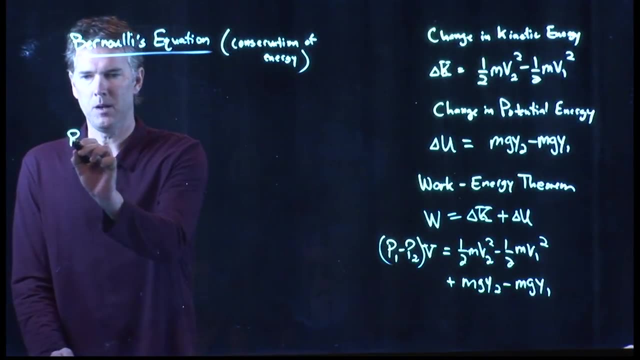 work is P1 minus P2 times V. That's one of the terms that we're going to need. Let's see if we can calculate the other terms that we're going to need and we'll put it all together. All right, let's separate the terms. We've got P1 times V. I'm going to move this V1. 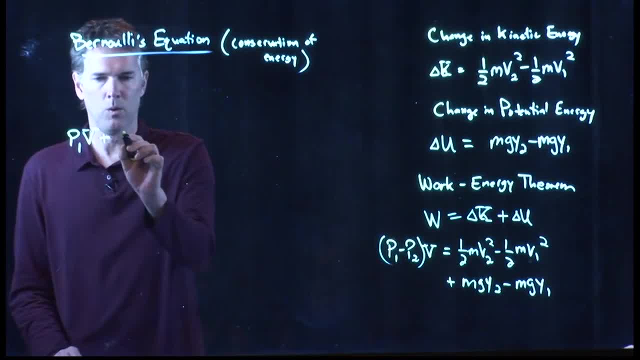 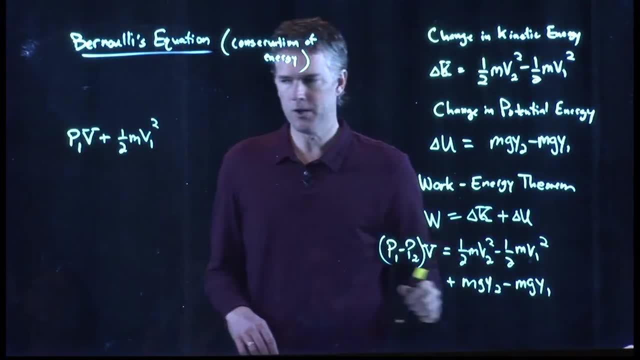 term over to the other side. so we have one-half m V1 squared, And now I'm going to move the Y1 term over the left side, so I have mgY1.. And now all the stuff on the right I want to leave as 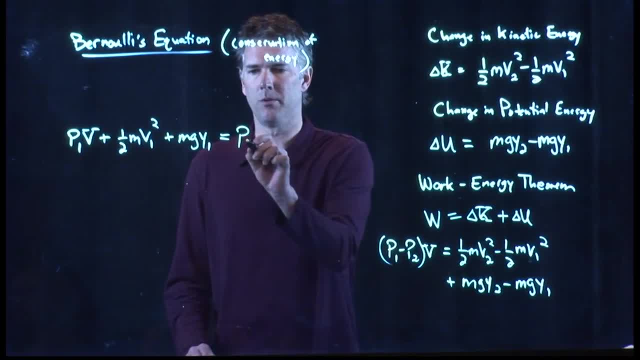 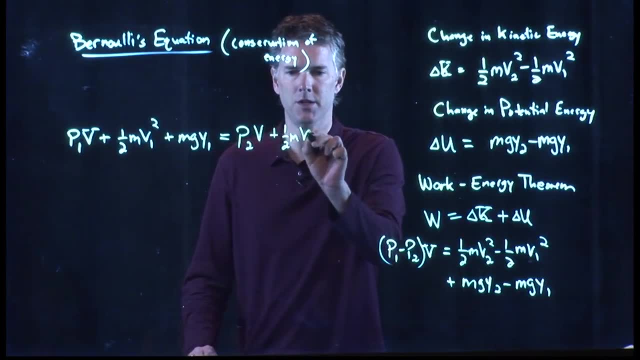 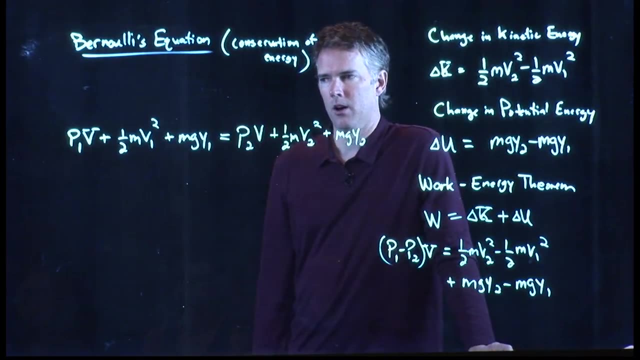 number two. so let's move P2 over to the right side And we have a one-half m V2 squared and we have an mgY2.. All right, that looks pretty good, except I don't really like this volume V. 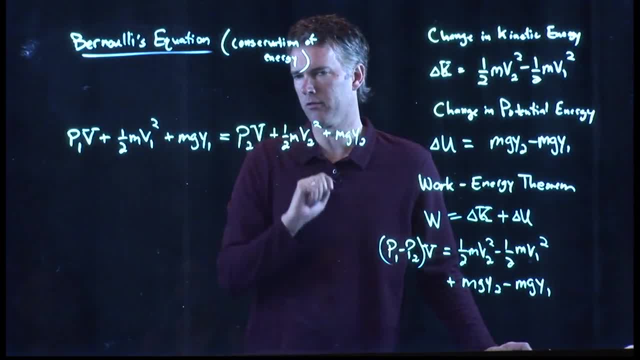 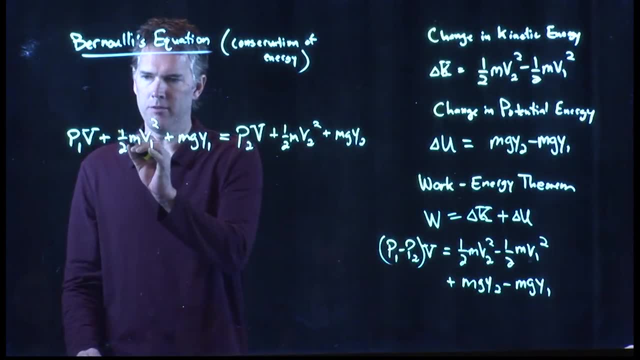 And I tried to write capital V and small v, because this one's a speed, this is a volume, So let's divide everything by V. If I divide everything by V, what's going to happen? That goes away. I put a capital V down. 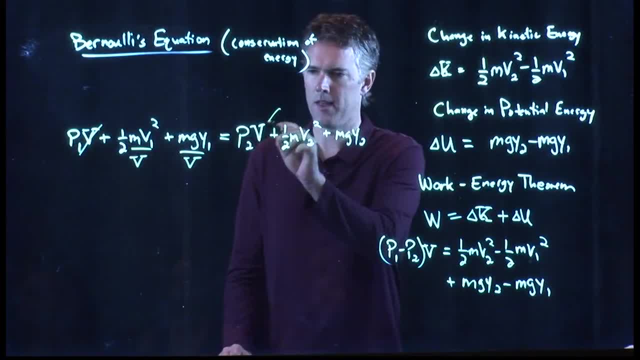 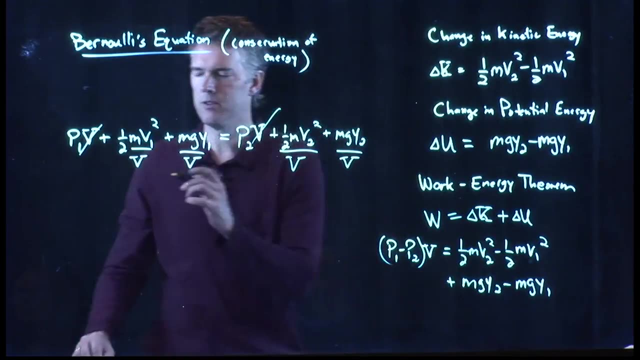 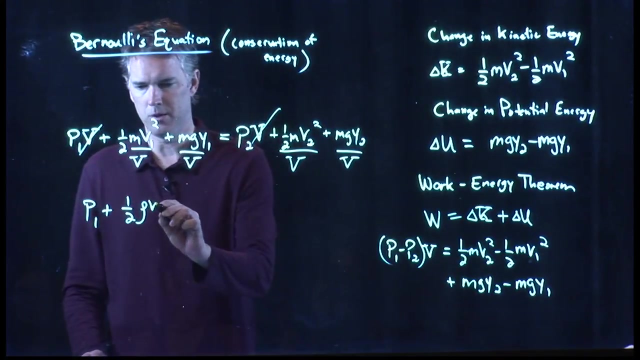 There. I put a capital V down there. That goes away. This, we put a capital V down there, and that we put a capital V down there, And that looks pretty good, because mass over volume is density, And so this becomes rho times V1 squared: Mass over volume, that's density.